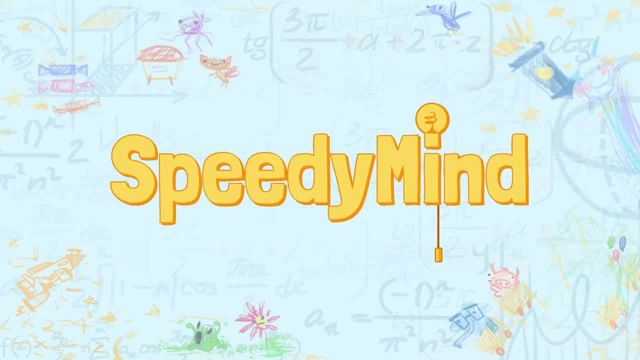 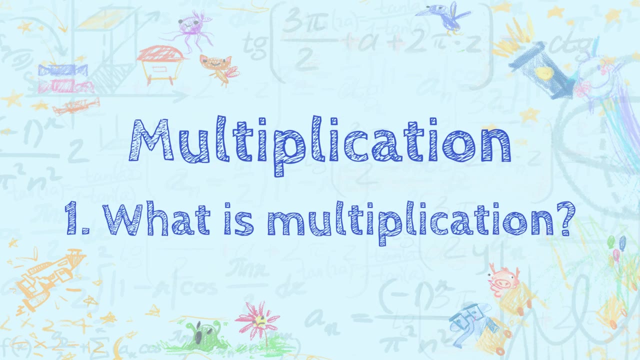 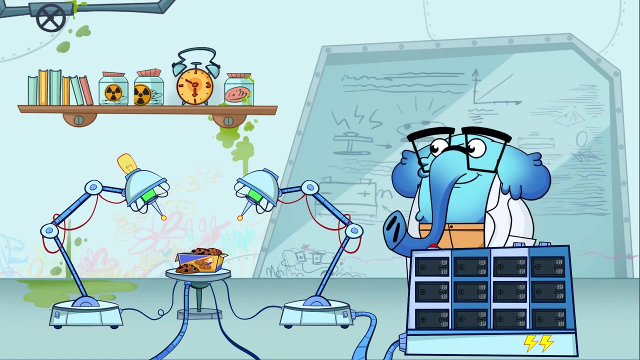 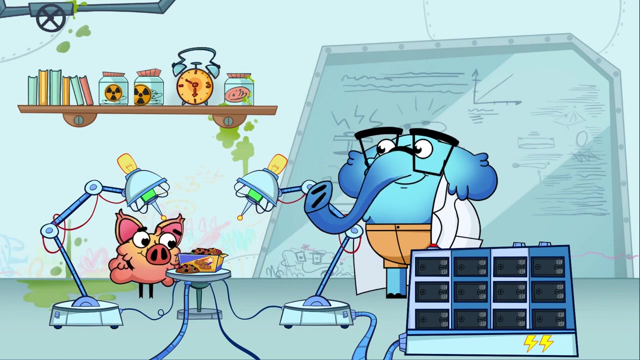 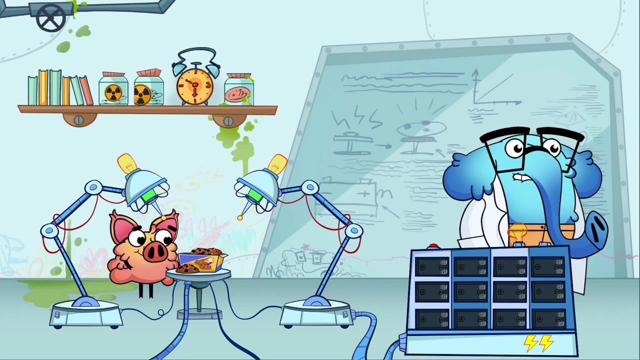 Thank you for watching. Oh, hello Piggy, Did you notice that the cookies in the package are too small? We run out of them every day. That's why I decided to invent a cookie enlarger. It will make them bigger and will have enough to last all day. 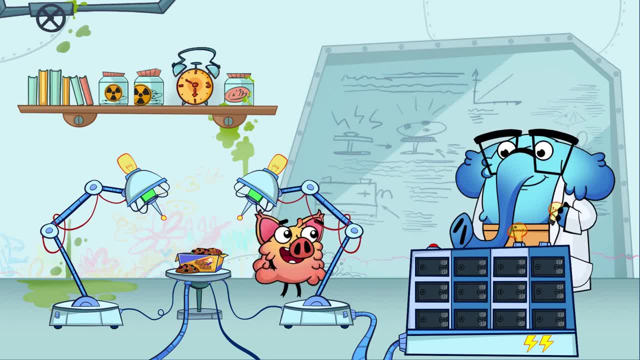 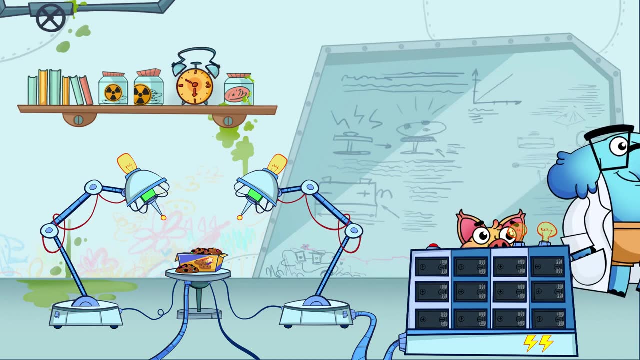 Wow, what a great idea. You know that I love sweets. By the way, I am almost finished with the device. The only thing left is to find the right size batteries. Let's go for a walk and look for some Sure, It's always so much fun being around you, Professor. 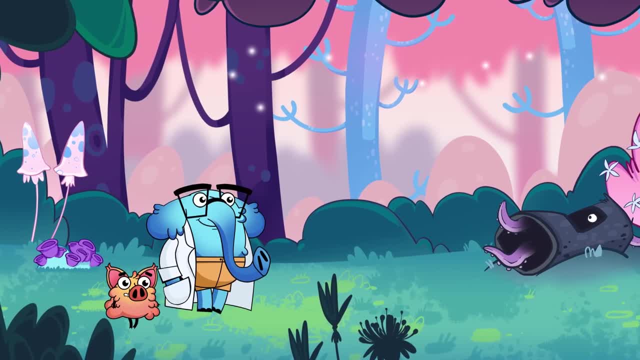 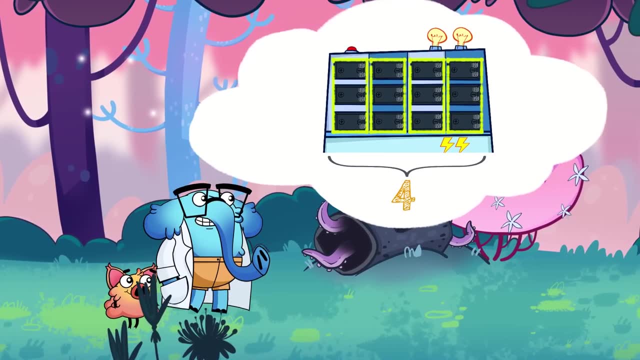 By the way, Professor, how many batteries do we need? Well, you can see that the device has four sections. It has three sections of batteries and each section holds three batteries. So if you multiply three by four, you'll get the answer. 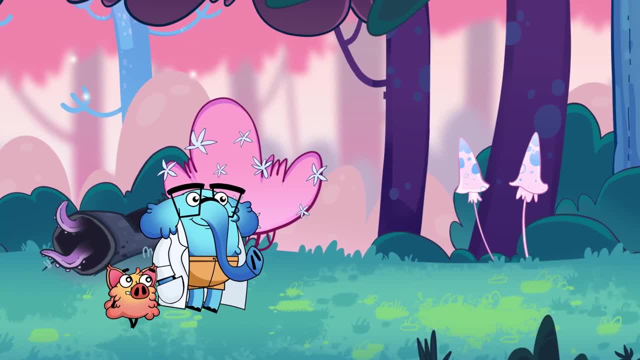 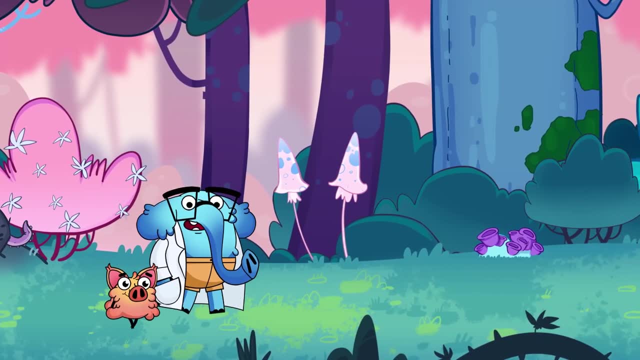 Hmm, What does multiply mean? I know how to add numbers, But if you multiply numbers, is that the same? Oh Piggy, don't worry, I didn't know that you haven't learned multiplication yet. Do you want me to explain how to multiply on our way? It's very simple. 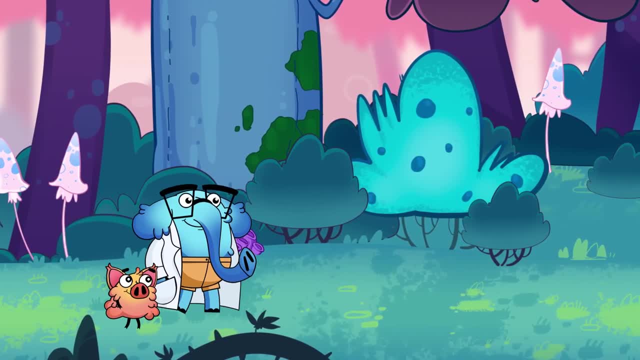 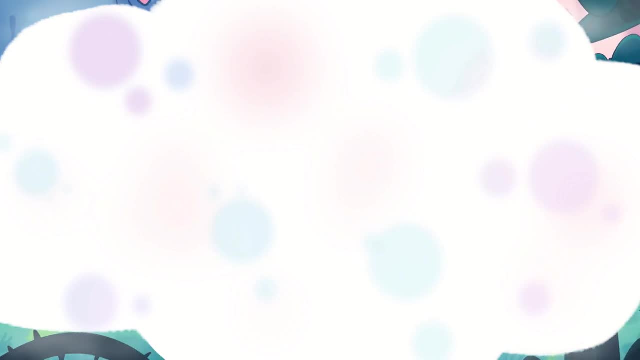 Sure thing, Professor, That will be wonderful. Well, you see, Piggy, when you multiply numbers, it's called multiplication. You already know that numbers can be added and subtracted, And now I just told you they can be multiplied too. 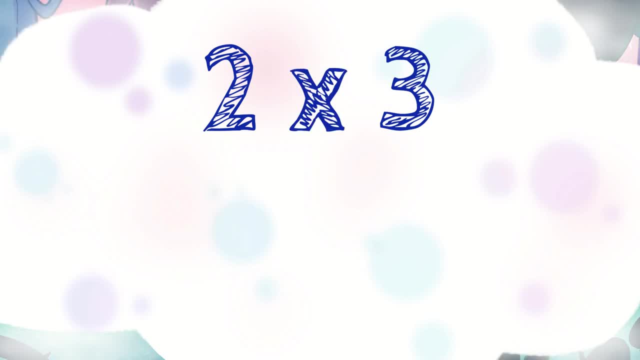 Multiplication is represented by the X symbol, and so we say two multiplied by three, or two times three. Multiplication means extended addition, And so we use multiplication to add the same numbers of items several times. The first number we multiply is the number of items in each group. 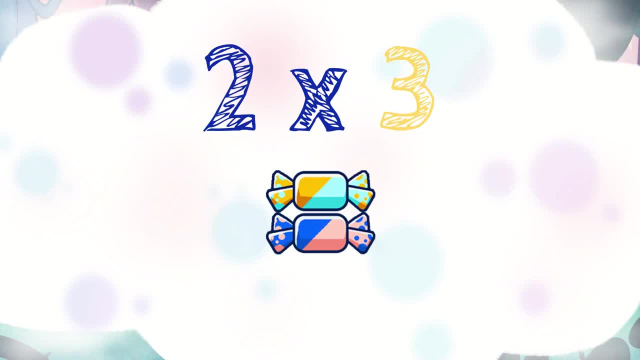 Let's say there are two pieces of candy in each group and the second number we multiply is the number of groups. So pretend there are three groups. So there are three groups of two pieces of candy each. How many pieces of candy are there in all? 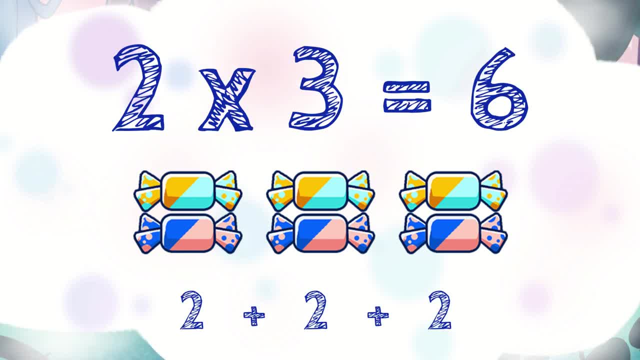 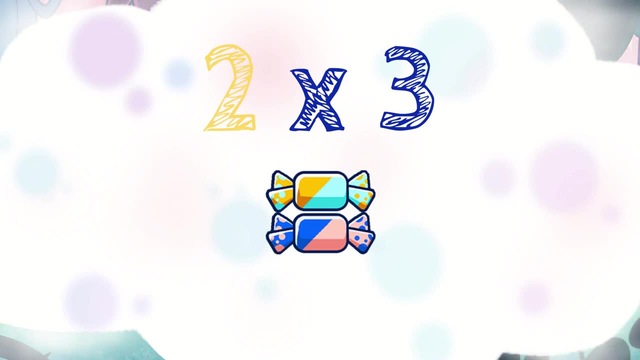 One is two plus two plus two, which makes six pieces of candy. So then, two times three makes six. Let's repeat this process one more time. The first number is the number of items in each group. The second number is the number of groups. 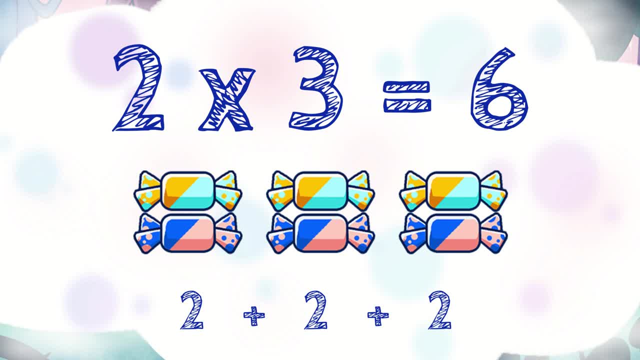 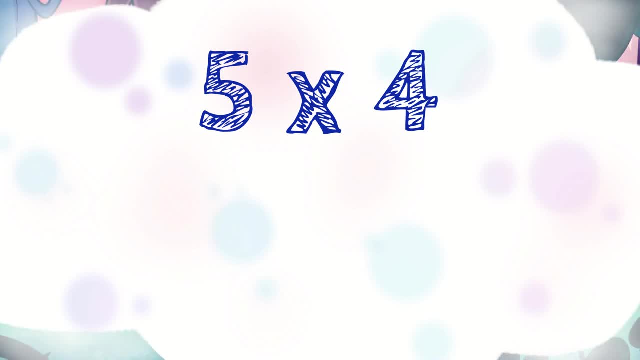 And the result of multiplication is the total number of items. Let's take another example: Five times four. The first number means the number of items in each group. So in this case we have five candies in each group. The second number is the number of groups. 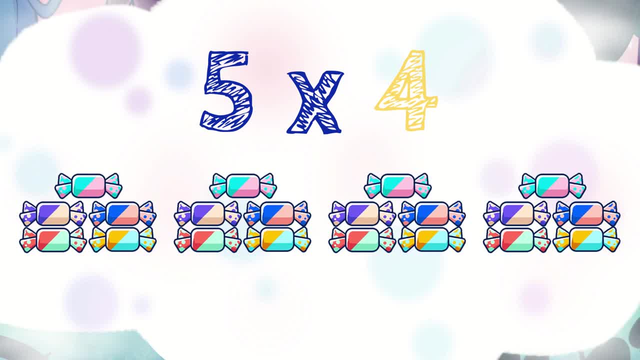 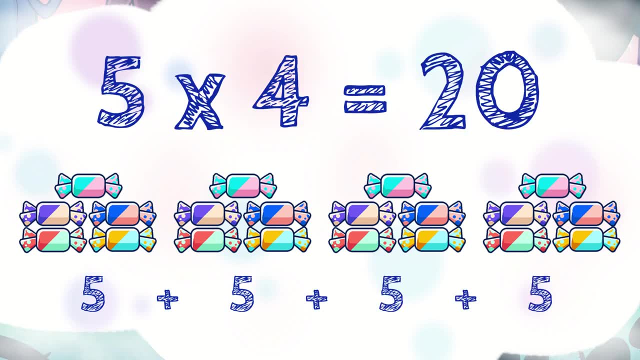 There are four groups of five candies. So then it will be five plus five plus five plus five, And there are twenty pieces of candy in all. So then, five times four is twenty. And now it's your turn, Piggy. 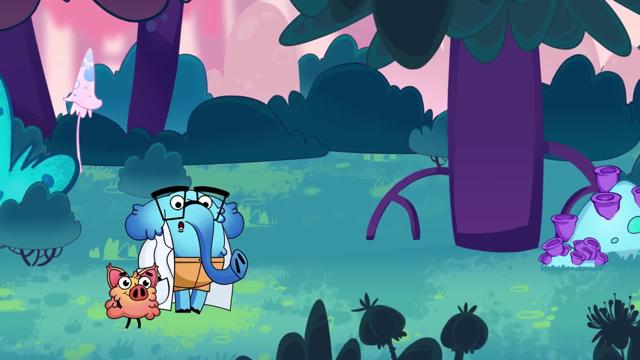 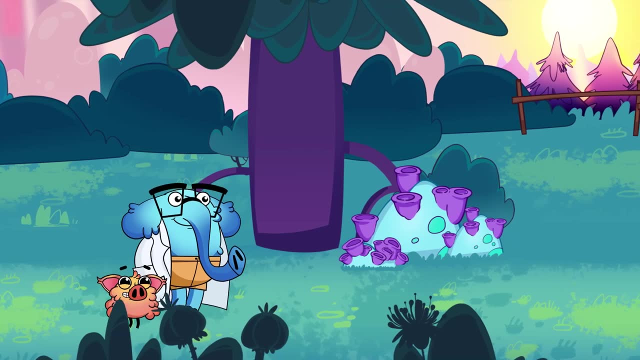 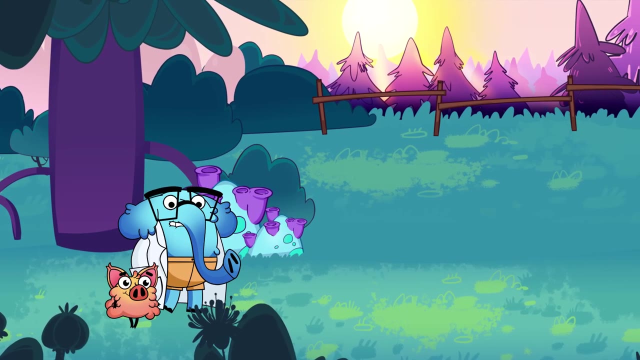 I know you can do it. How much is four times two? Can I count using ice cream cones, Professor? Yum, I like ice cream even more than candy. Sure Piggy, It doesn't matter what you count, The answer will always be the same. 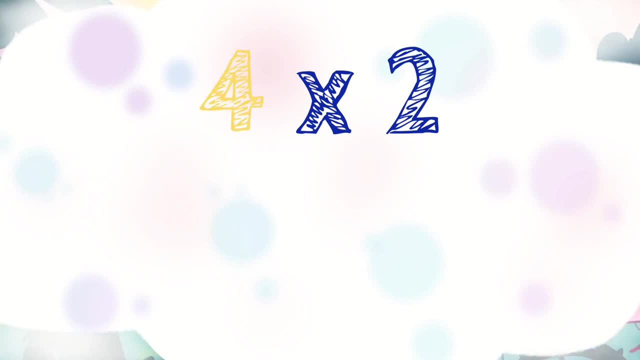 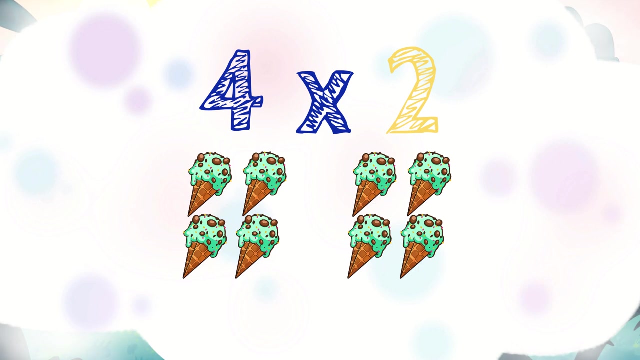 So the first number is the number of ice cream cones in each group. That means we have four ice cream cones in each group. The second number is the number of groups, And there are two groups of ice cream cones. In total, that's four plus four ice cream cones. 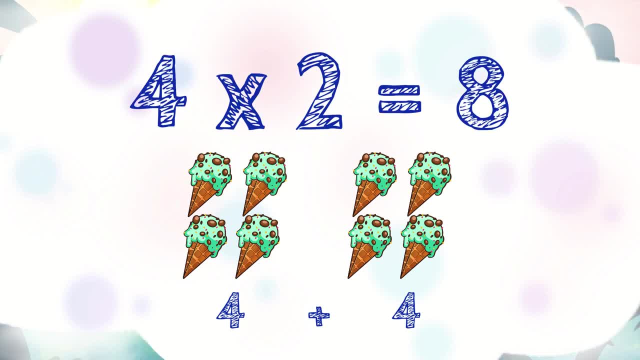 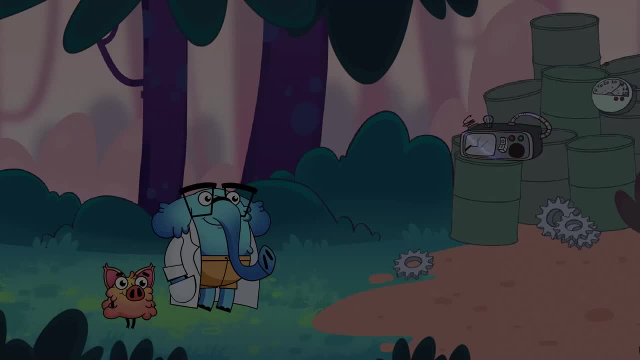 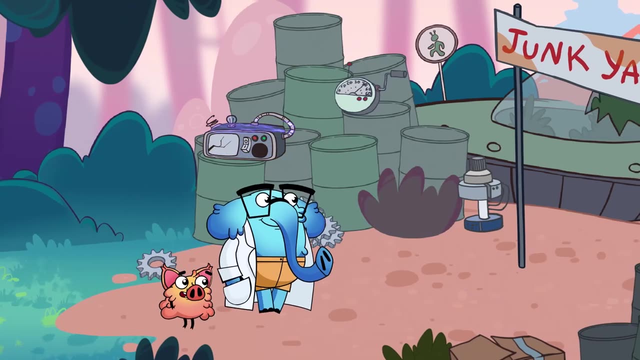 And that is eight, Which means four times two is eight. You're right, Piggy. Excellent job, Piggy. it looks like we've arrived, Professor, are we looking for batteries in a junkyard? Yes, Everything here is free. 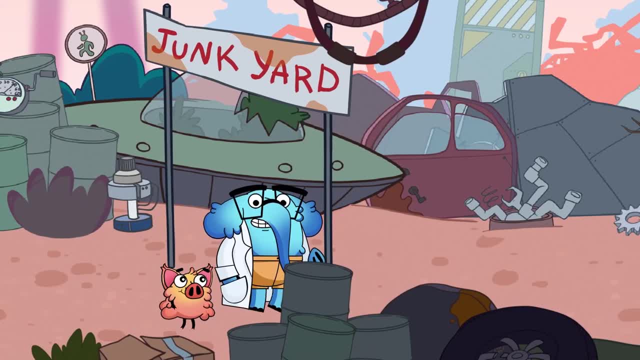 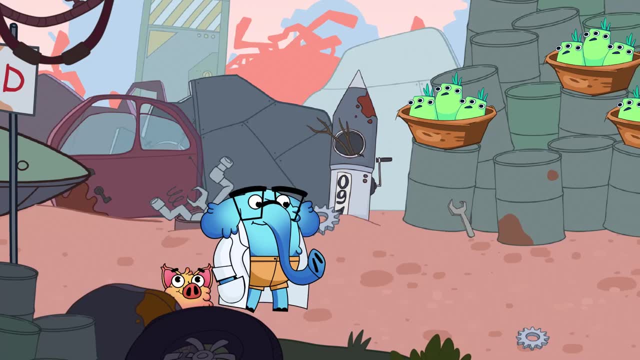 And also, there's no sense buying new things when we can reuse old ones that still work. While we're looking for batteries, let's find some examples that we can use multiplication for around here. Hey Piggy, check out these bird nests. 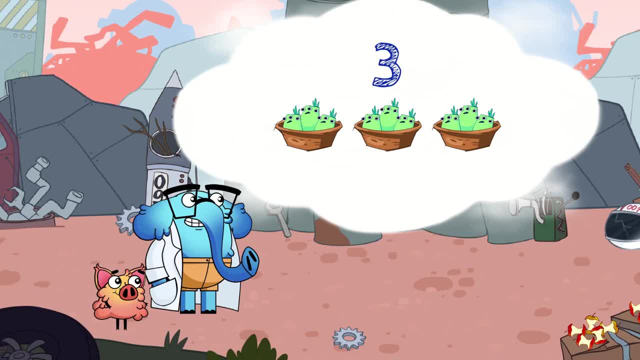 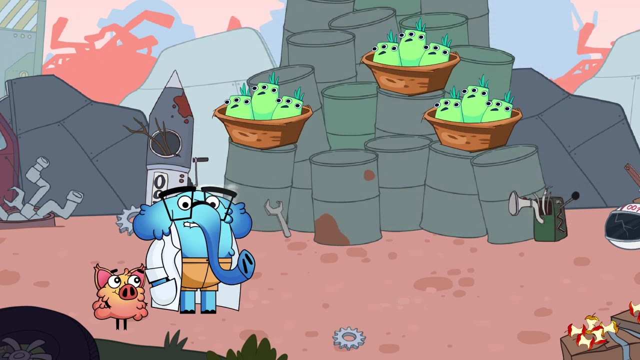 There are three birds in each nest And there are three nests, So that would be three times three. There are three plus three plus three birds, For a total of nine birds. Now it's your turn, Piggy. What can you find? 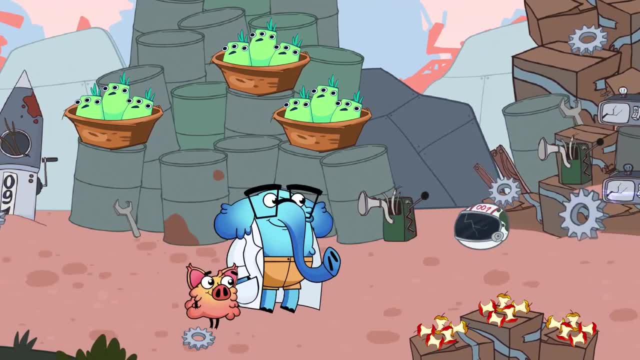 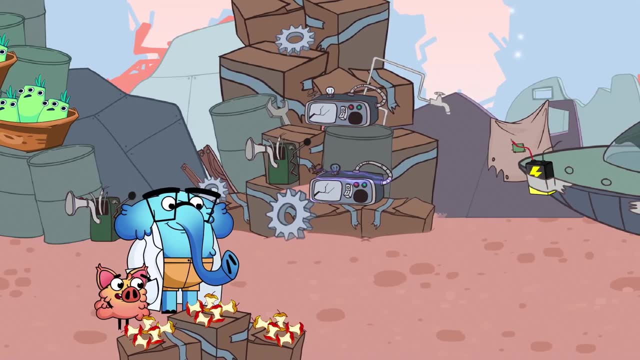 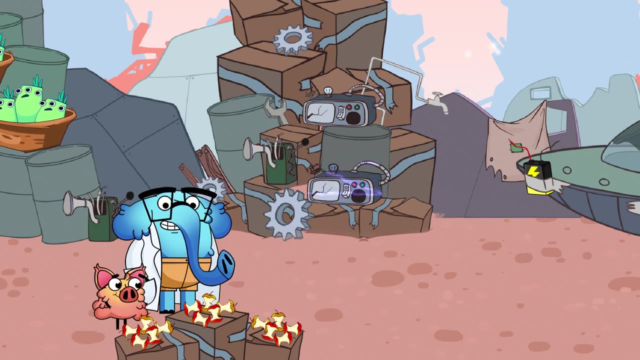 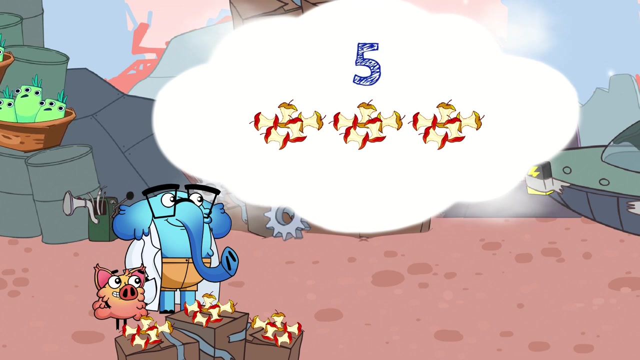 Let me see. Wow, I think I have found my example, Professor. Look, Three piles of five apple cores each. Good example, Piggy. Now how will you write this using multiplication? Hmm, I know. Five apple cores in each pile. 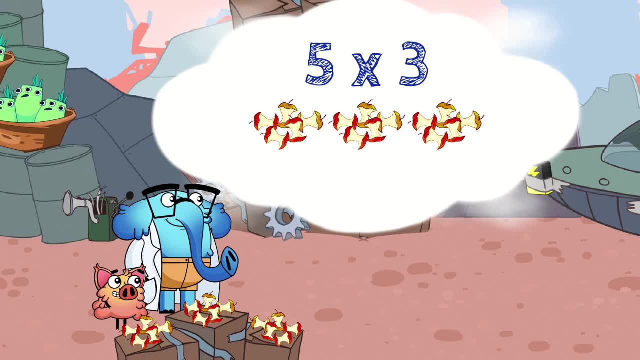 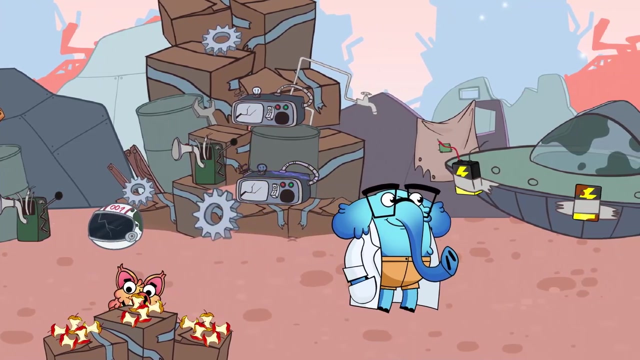 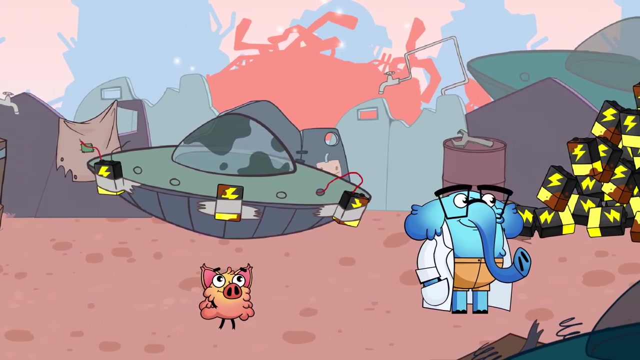 And there are three piles, So that will be five times three. There are five plus five plus five apple cores. in all That makes fifteen. So five multiplied by three is fifteen. Great job, Piggy. Hey, I just found some batteries. 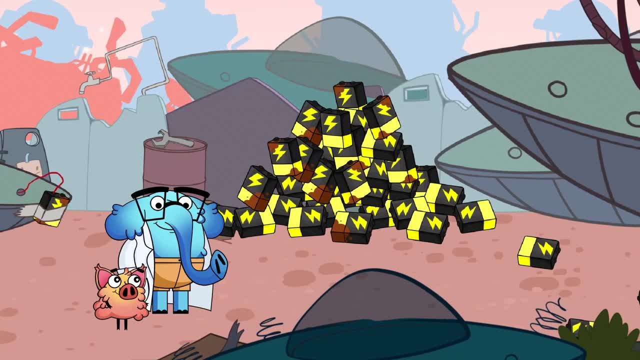 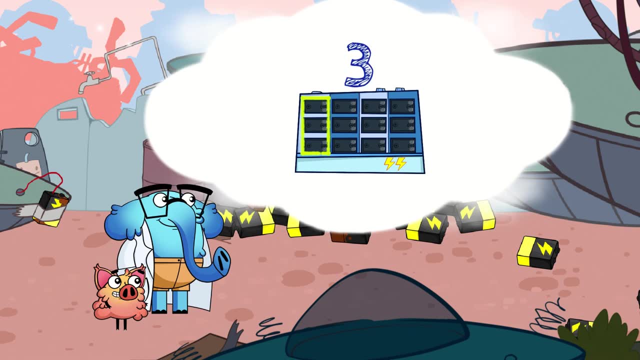 Piggy. how many batteries do we need? Can you count using multiplication now? Hmm, Let's see Three batteries in each section And there are four sections. So that would be three times four, And that is three plus three plus three plus three. 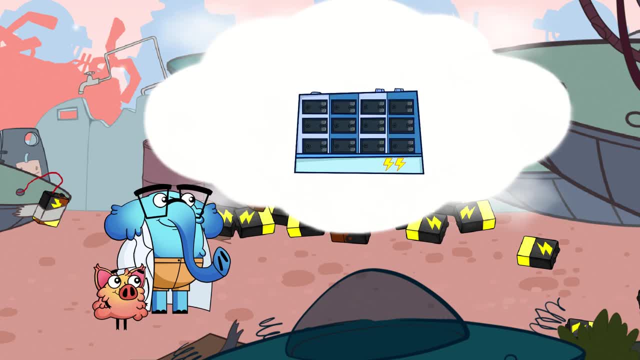 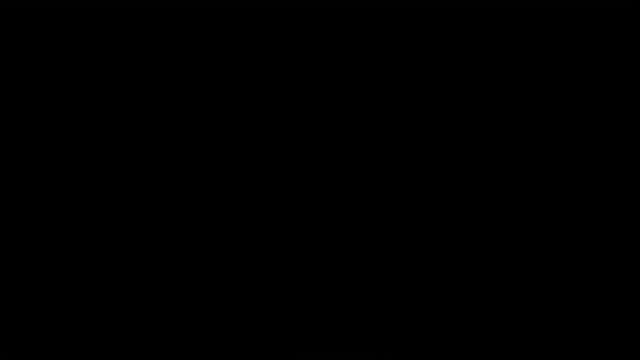 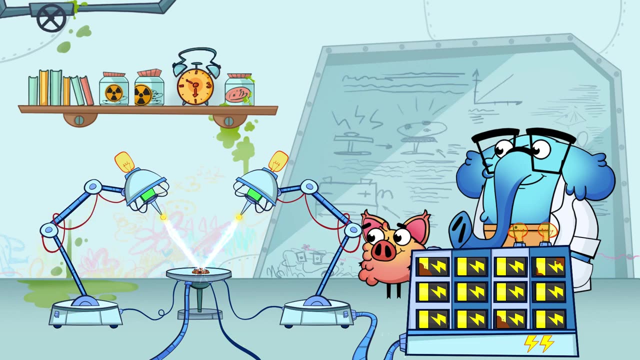 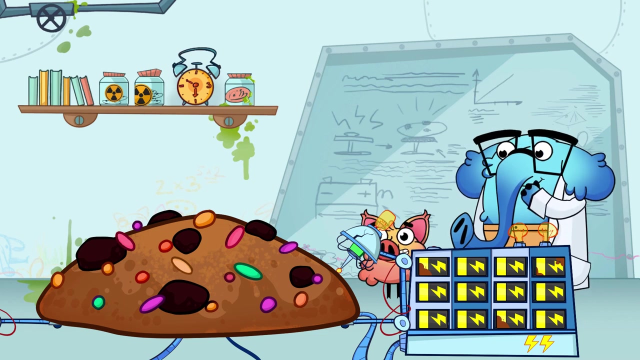 Twelve batteries? Absolutely. Let's pick them up and go home to try out our device. Everything is ready. Let's see if it works. Yes, We did it. Yummy, Ah, Our device definitely works. I think now we can take a break and drink some milk with our cookies.